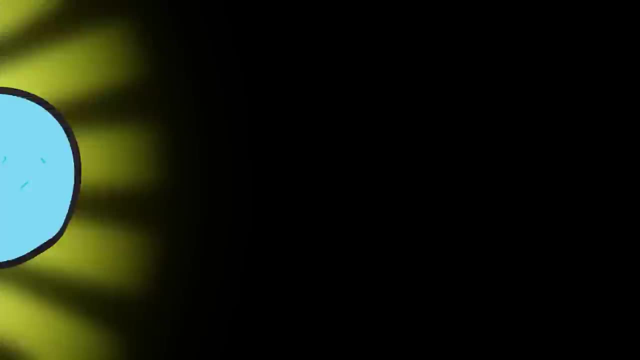 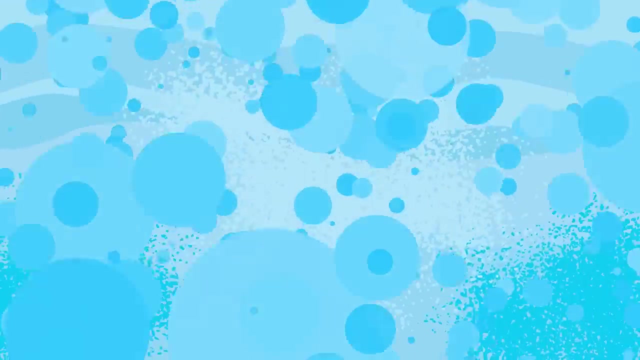 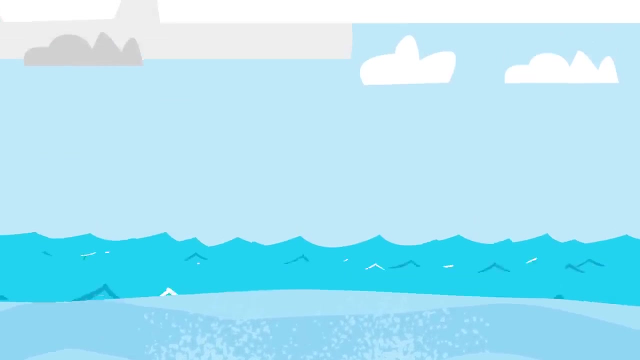 darkness. God called the light day and the darkness night. On the second day, God said: Let there be a space to separate the waters of the heavens from the waters of the earth. God called the space sky. On the third day, God said: 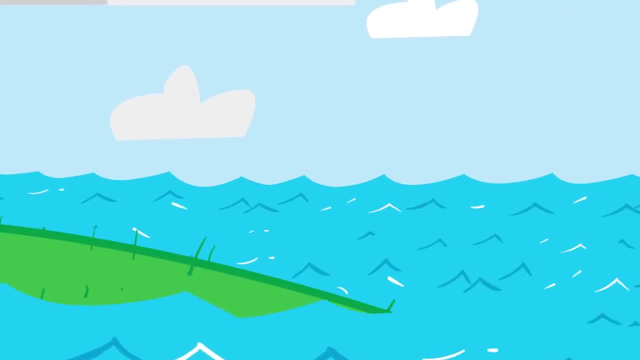 Let the waters beneath the sky flow together into one place, so dry ground may flow. God called the dry ground land and the waters seas, And God saw that it was good. Then God said: Let the land sprout with every sort of plant and tree. 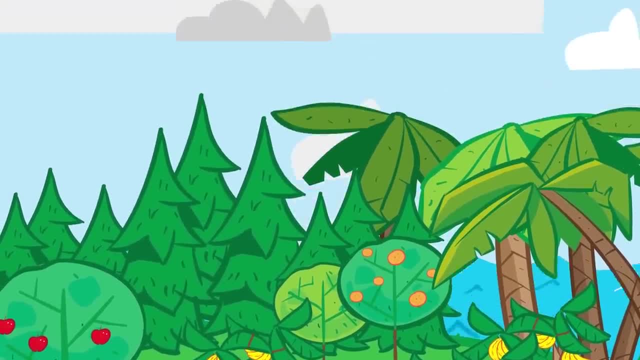 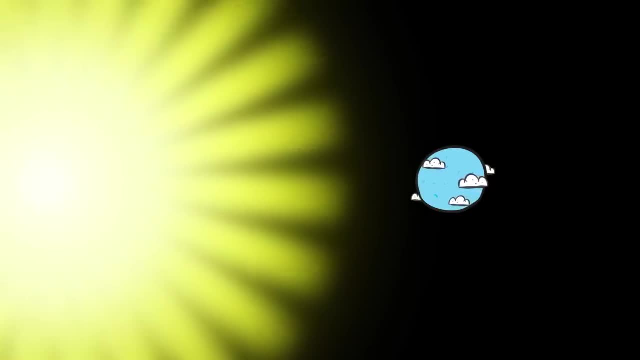 And God saw that it was good. On the fourth day, God said: Let lights appear in the sky to separate the day from the night. God made two great lights: the sun for the day and the night for the night. God made two great lights. 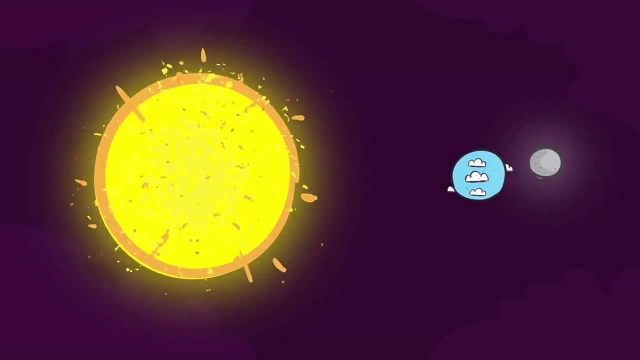 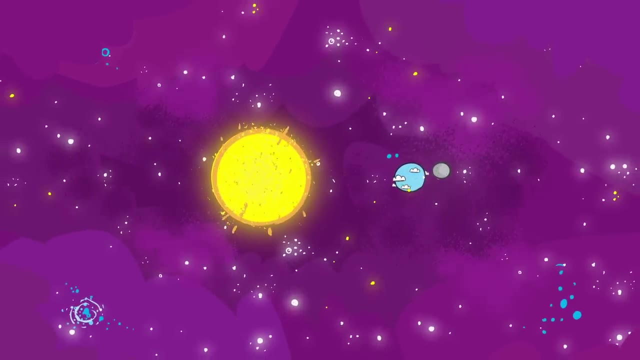 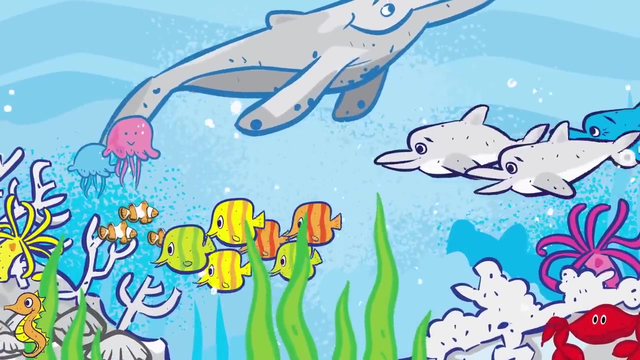 and the moon for the night. he also made the stars. God set these lights in the sky to light the earth, and God saw that it was good. on the fifth day God said: let the water swarm with fish and other life. let the skies be filled with birds. 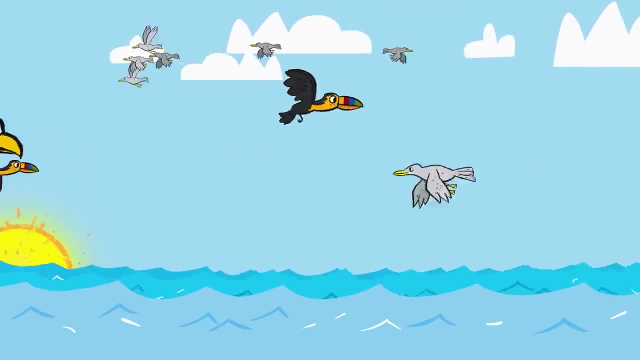 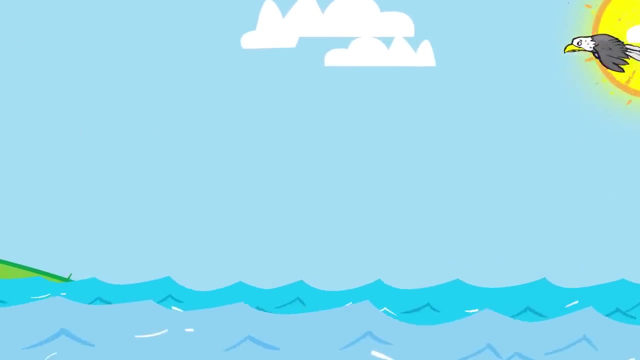 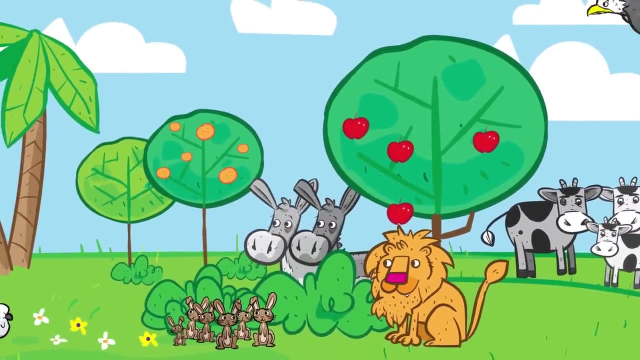 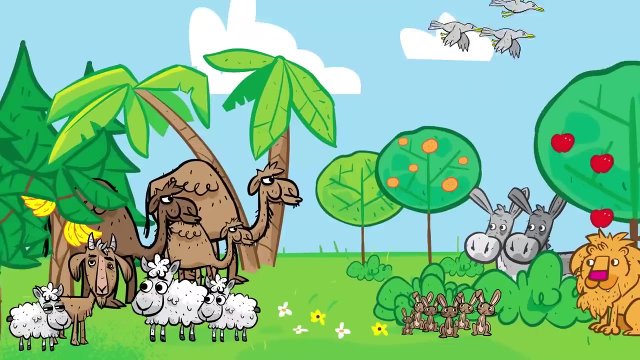 of every kind, and God saw that it was good. on the sixth day God said: let the earth make every sort of animal. God made all sorts of wild animals, livestock and small animals, each able to have babies of the same kind, and God saw that it was good. then God said: let us make man in our image, to be like us. 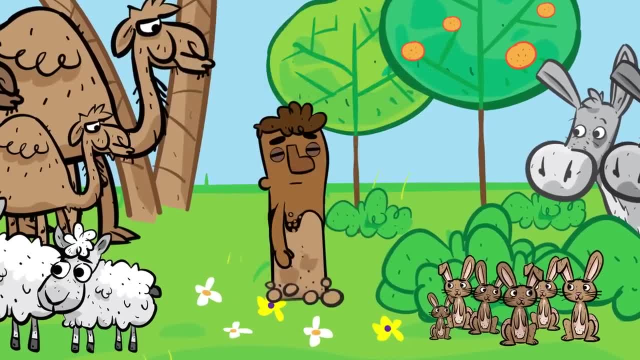 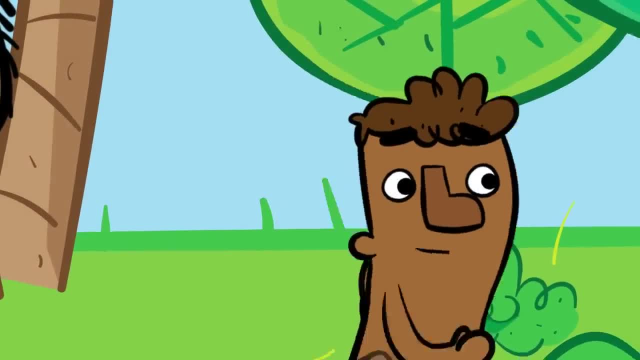 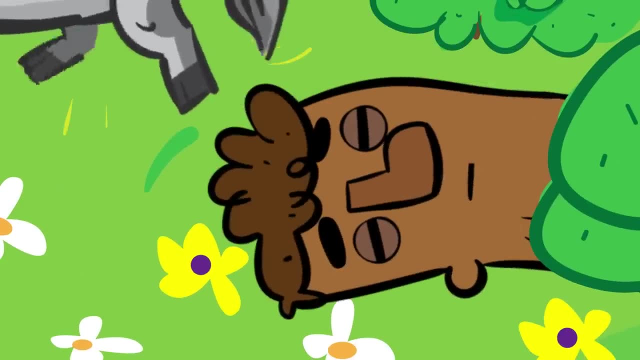 you. so God created man in his own image. he formed man from the dust of the ground. he breathed the breath of life into man, and a man became alive. then he saw that the man needed a helper. so God put man into a deep sleep and while he slept, 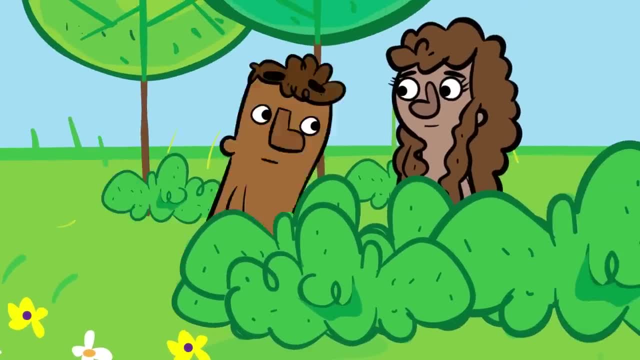 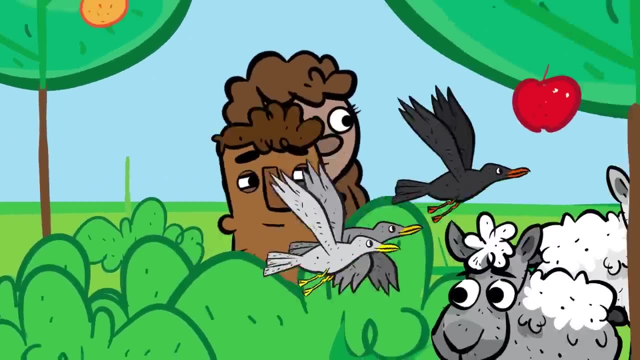 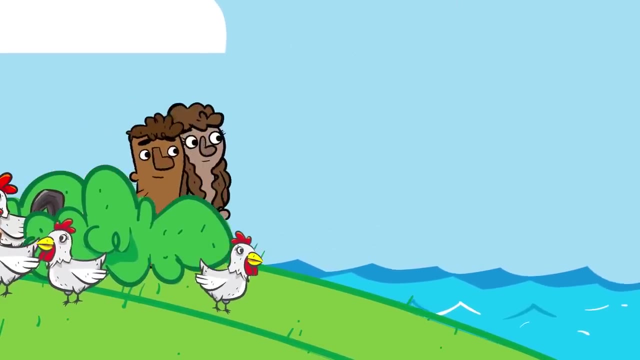 God took one of the man's ribs. then God made a woman from the rib and brought her to the man. then God's bless them and said: be fruitful and multiply, fill the earth and rule over it, Rule over the fish in the sea.